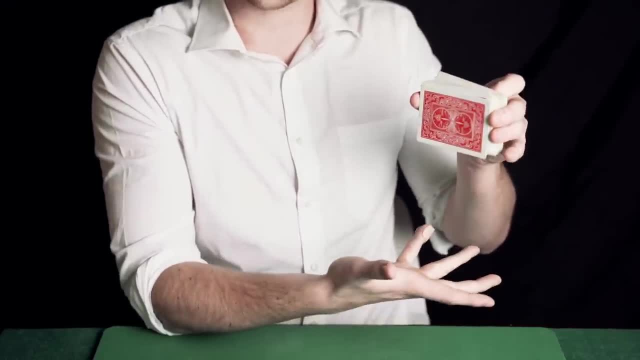 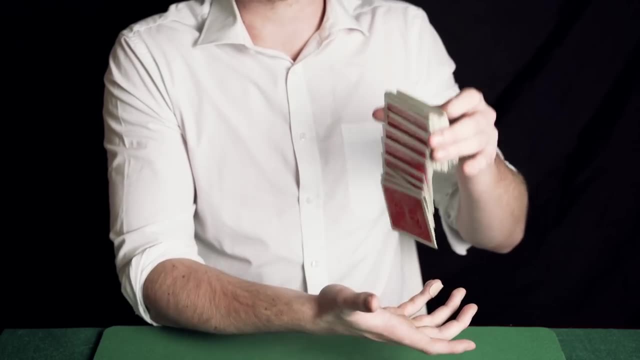 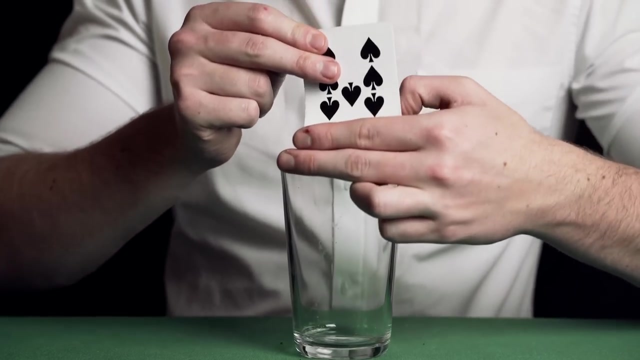 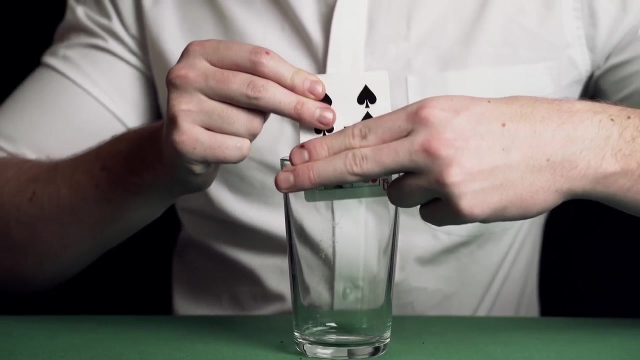 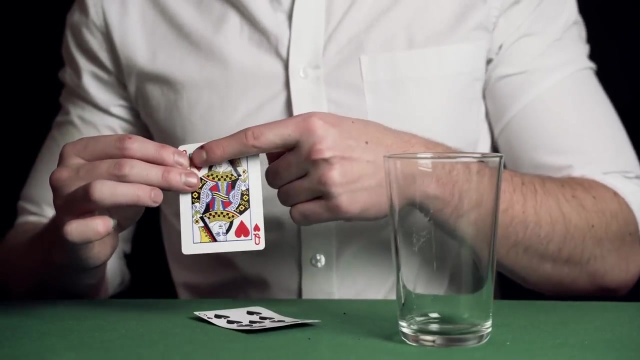 fall into your hand. So you just do this all in one movement and you can really create the illusion that you're a professional magician with these cards. The card slowly and visually changes. In order to do this trick you need two cards, Put a piece of double sided tape or 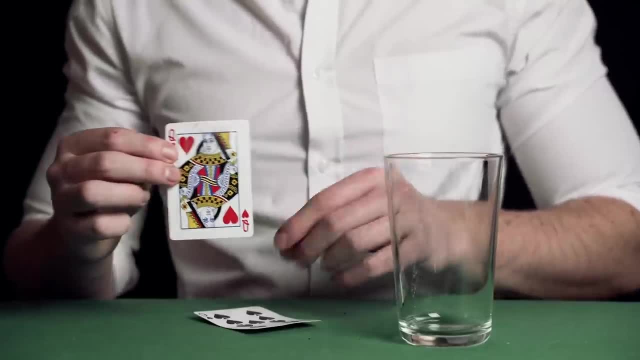 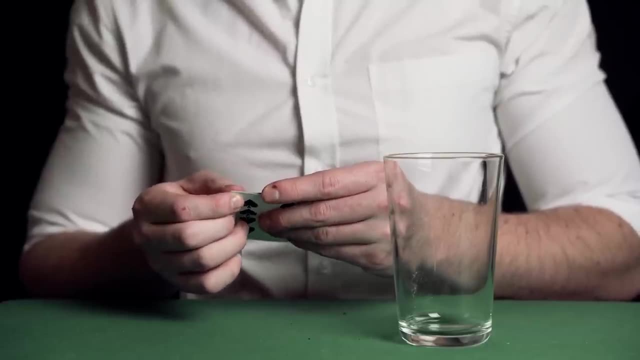 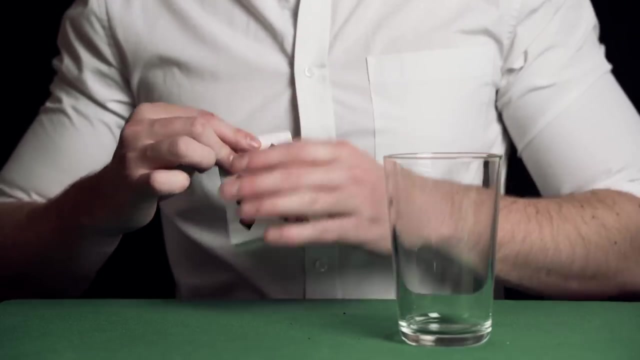 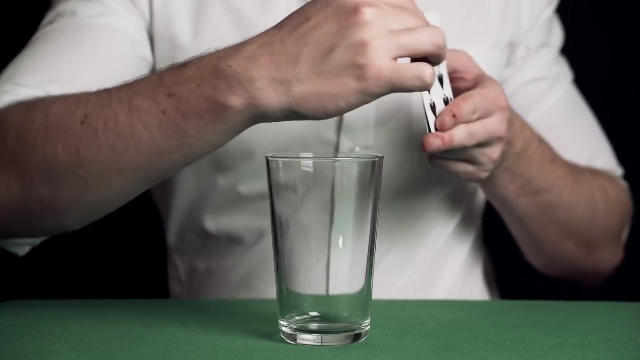 sellotape wrapped over twice on top of one card and then place the other card on top and align up the edges. perfectly. This creates a flap system. now what you need to do is have a glass, so show the card as single and then come over, and all you're doing is grabbing onto the card with your middle finger. 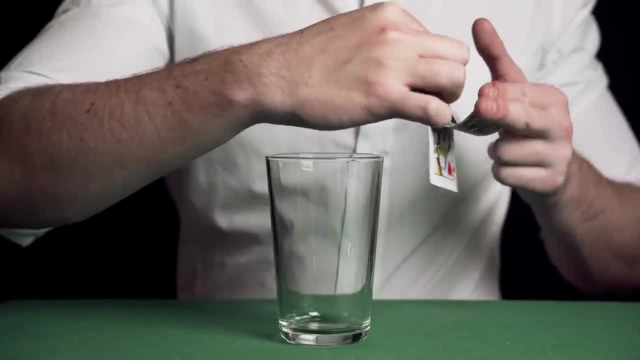 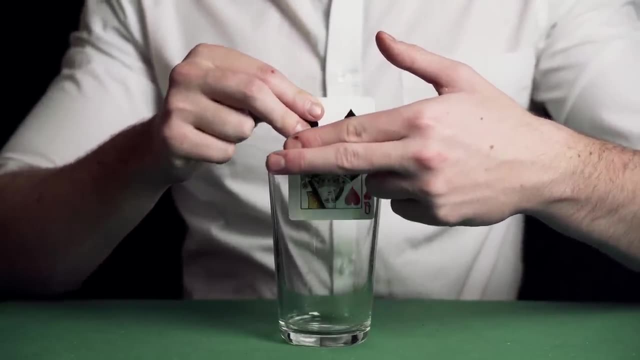 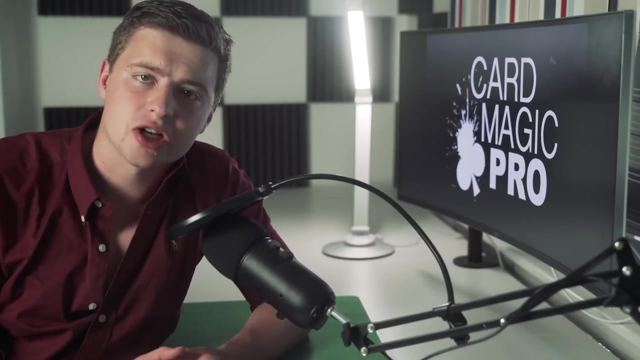 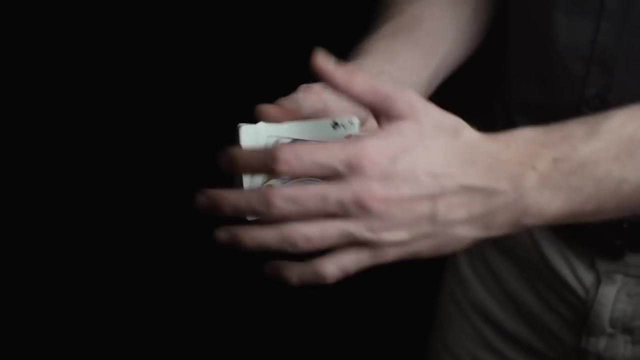 and pushing it down and, as you can see, this reveals the card behind, but from the front point of view, it looks as if the card has magically changed. If you're interested in learning incredible card tricks, including flourishes, cuts, shuffles and more, and tricks that are just too good to reveal on YouTube, then check out my magic. 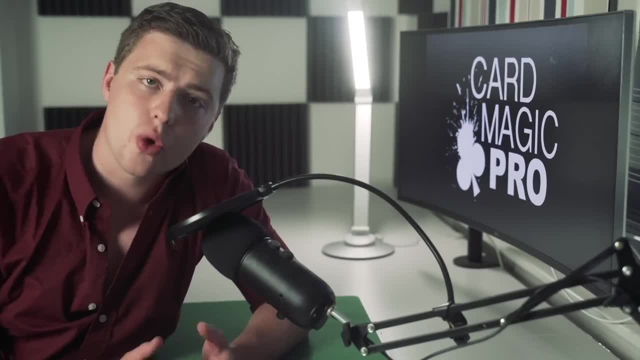 card course in the first link in the description below. The course contains some of the best tricks ever created and will give you the ability to walk into a room and impress anybody that you like. So go and check out Card Magic Pro in the first link in the description. 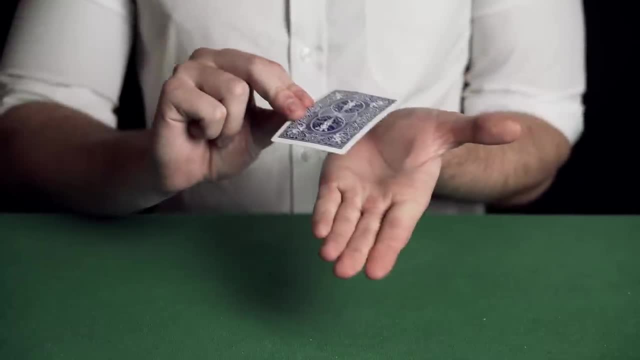 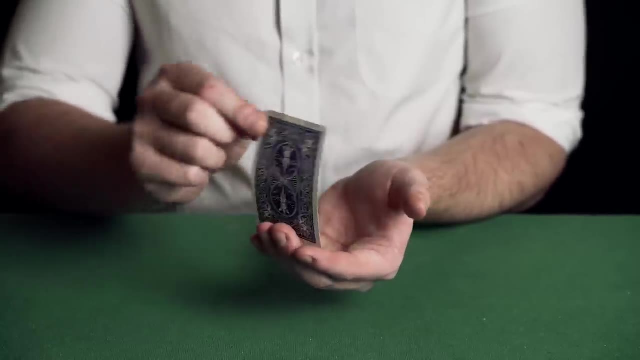 A card appears from nowhere In the first link in the description, the card will pop upwards. Take a card and place it into your open hand. Keep your fingers closed and use them to bevel the card towards you. When you release pressure with your palm, the card will pop upwards. 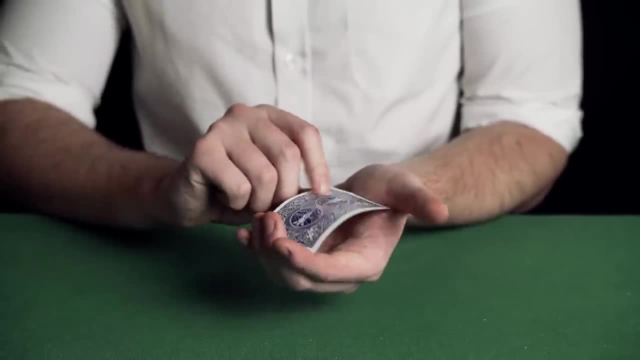 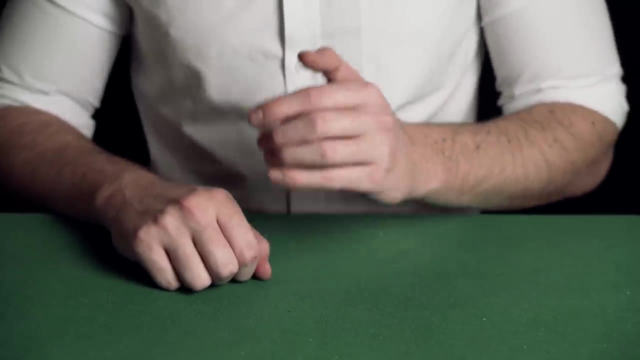 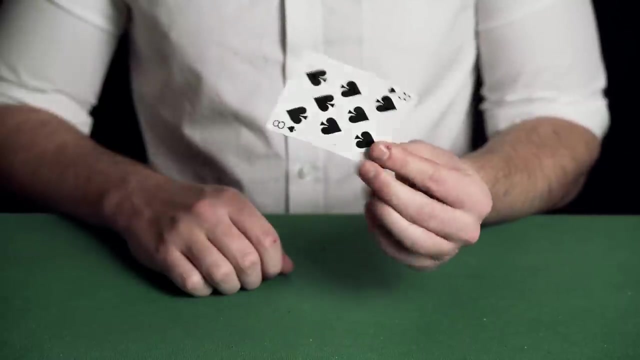 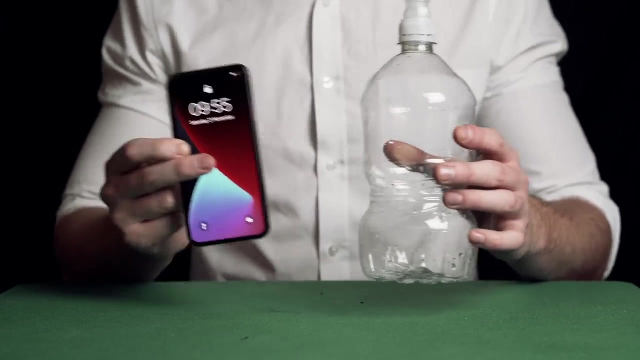 Catch the card between your fingers and thumb, as it appears. This will create the deceptive illusion that the card appeared from thin air. Now turn your hand. palm down. As you turn it, palm up. produce the card. pop upwards card. this is very visual. the magician has a phone in a bottle. he pushes the. 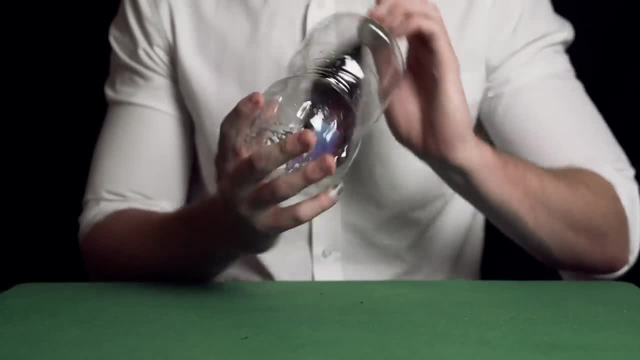 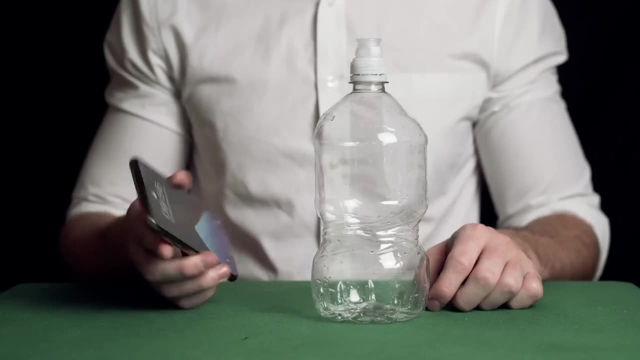 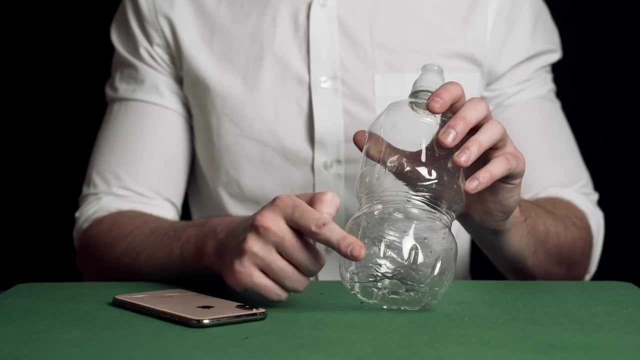 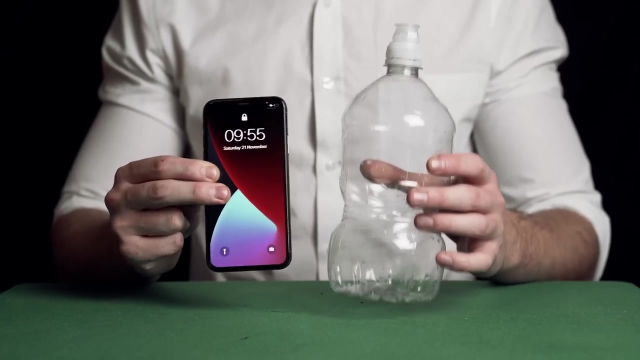 phone right inside the bottle. the phone is stuck inside. the secret behind this effect is very simple: simply cut giant slit in the side of the bottle with a knife, make sure your spectator is in front of you and then turn the slit so it's facing your phone. this way, they won't see it. now push the phone through. 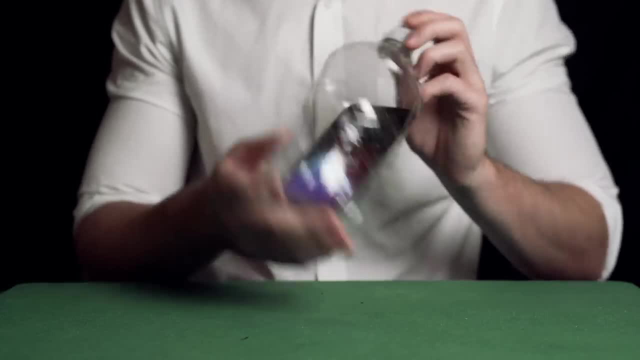 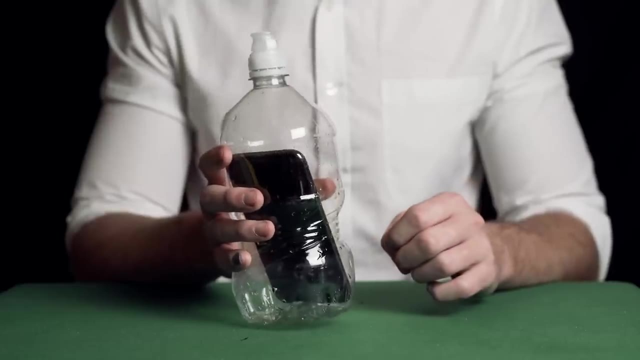 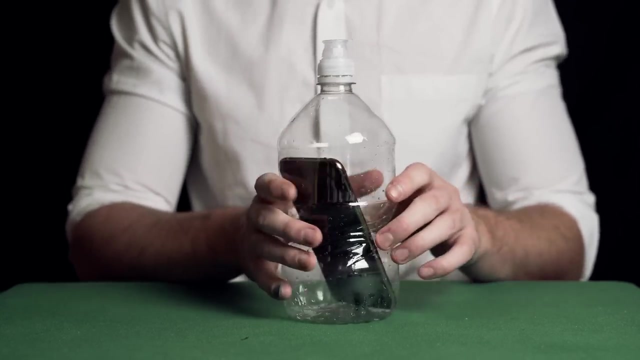 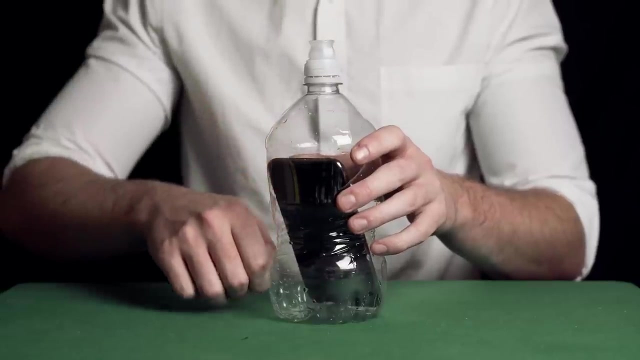 the slit, show that it's really in there, then say that you want to get the phone out and take a knife and pretend to cut into the bottle, but really all you're doing is just putting the knife through the existing slit. this way you can open up the bottle and remove their phone and end completely clean. they. 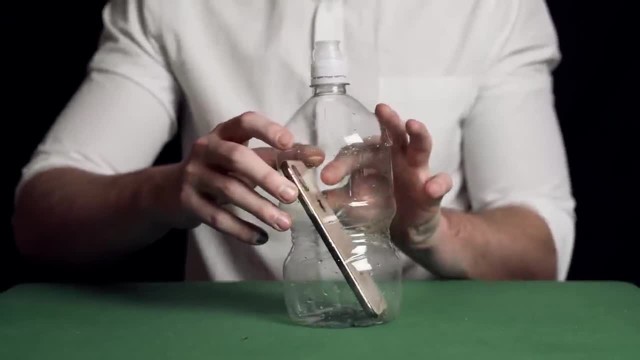 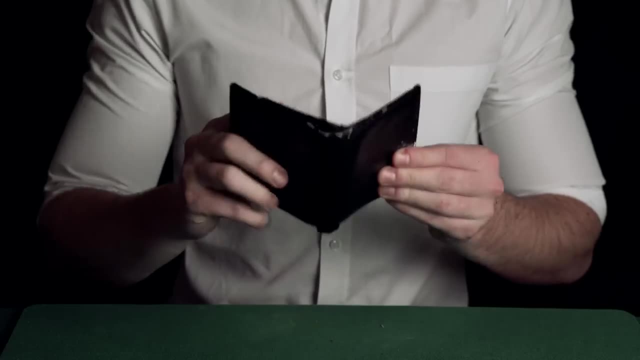 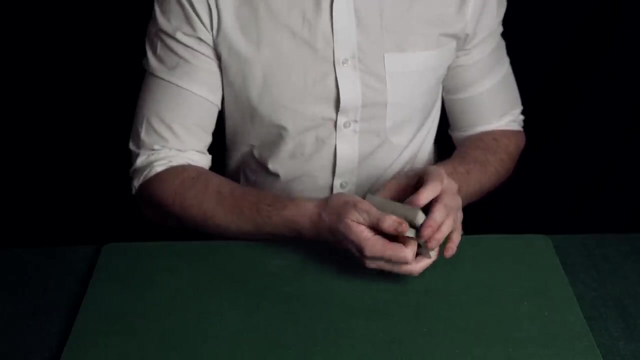 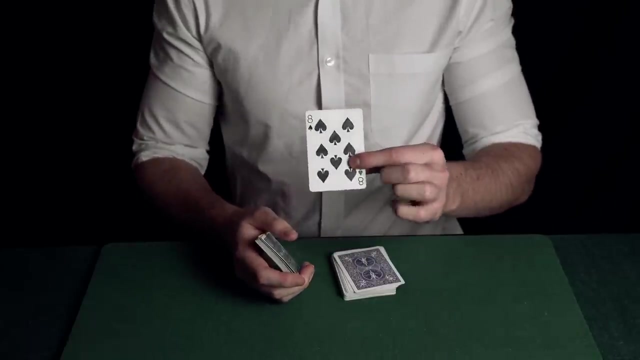 won't ask to inspect the bottle before the trick because they don't know what's about to happen. the magician's wallet bursts into flames. here is the same effect, but in a full trick. the magician shows. all the cards are different. he then tells the spectator to say stop and take his card. in this case it's the eight of spades. 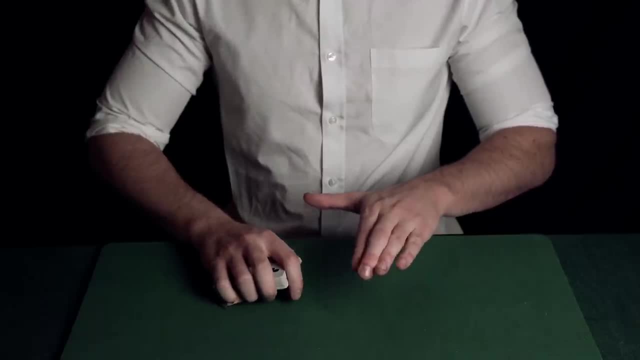 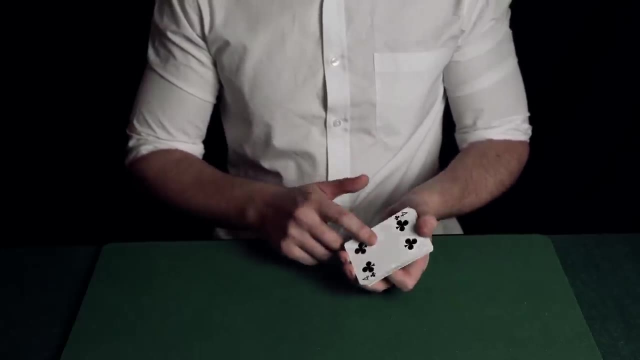 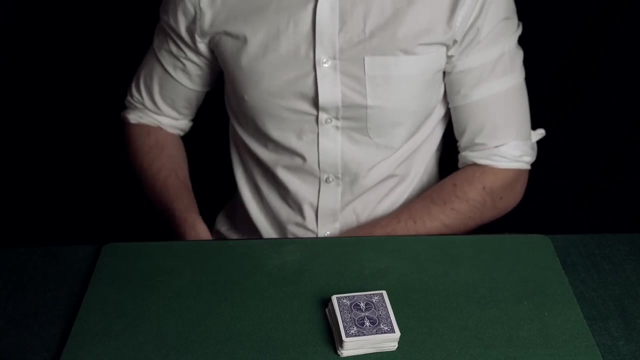 the magician rubs the eight into the table and it vanishes. it's not on the top of the deck, nor is it on the bottom. the magician then points to his wallet, saying that the card has jumped there. he opens his wallet and it bursts into flame. 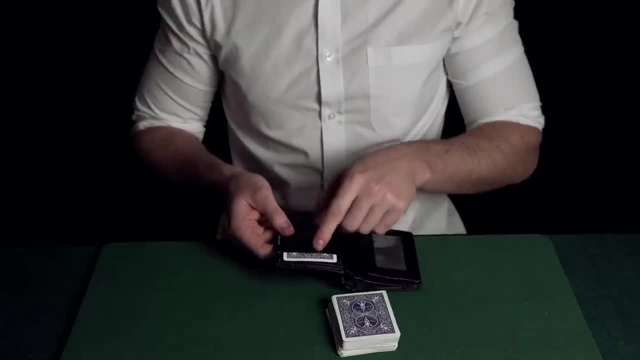 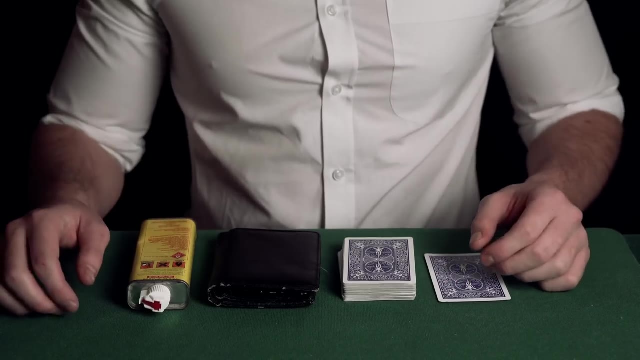 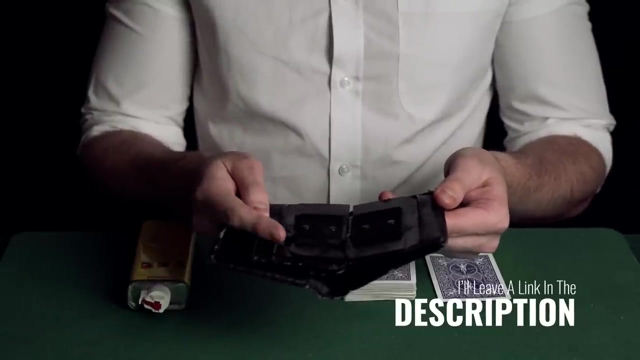 the flames suddenly disappear and inside the wallet, it's the spectator's eight of spades. this is one of my absolute favorite tricks to do. what you're going to need is a fire wallet. you can buy these on the internet and essentially, they allow you to pull this trigger. 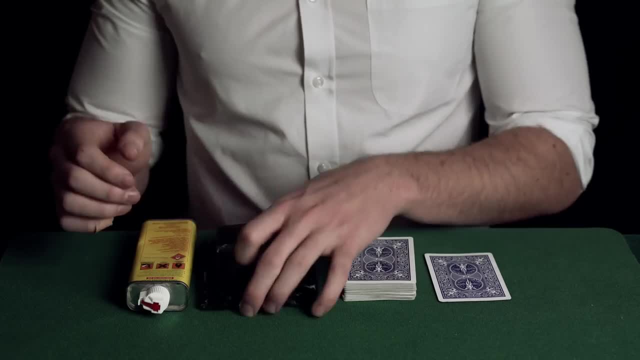 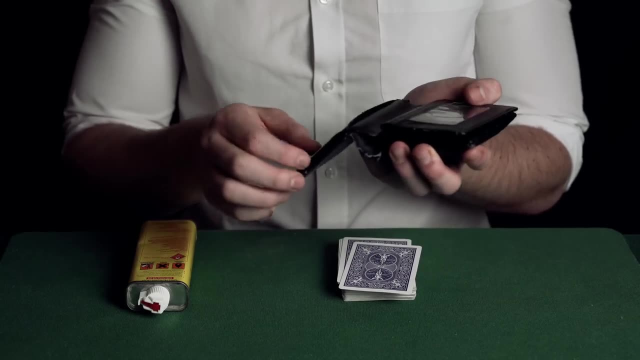 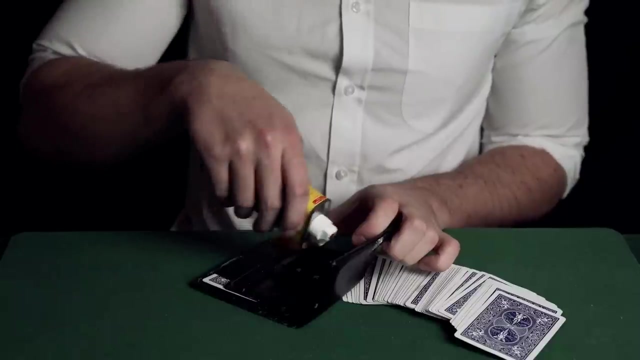 here and fire appears in the wallet, and what you also need is a normal deck of cards with a duplicate. so put the duplicate into the fire wallet like this and then put some of the cards- some lighter fluid- into the pouch in the fire wallet here. so you pull that in there. i've already. 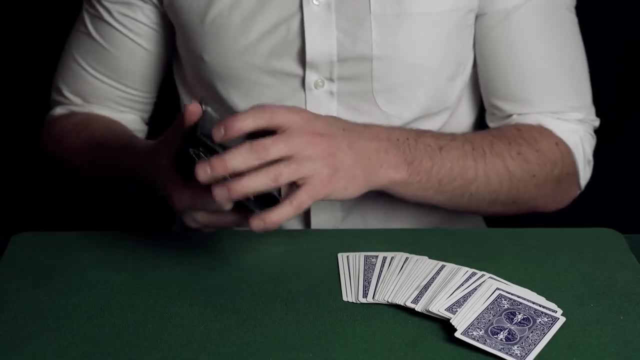 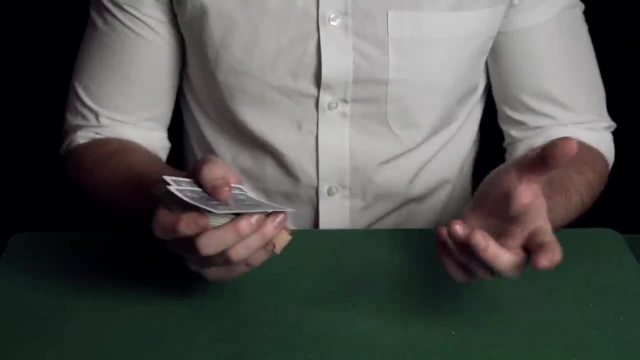 done it, so i'm not doing it now. and then you're ready to begin, so put the wallet in your pocket, so the first thing you need to do is force the spectator to pick the eight of spades. there are loads of ways to do this, loads of tutorials on the internet already, so i won't delve into them now. 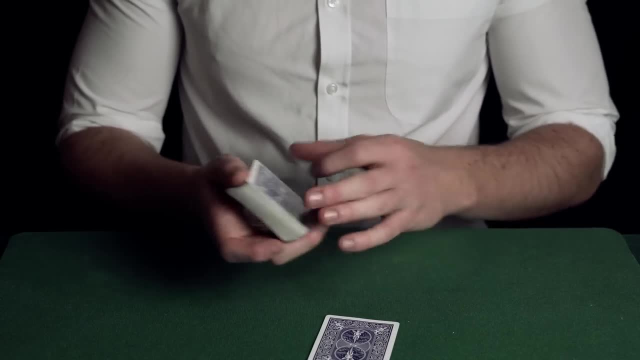 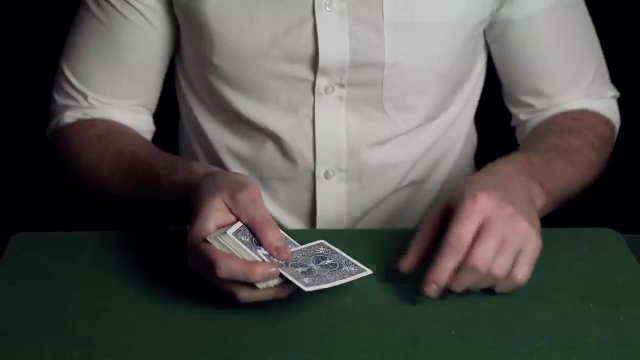 but make sure your spectator chooses the eight of spades. once they've done that, you need to make the card vanish again. you can do this any way you want, but the way i did it was you can do it using a retention vanish or a rubber dub vanish, so you slide your hand over the card. 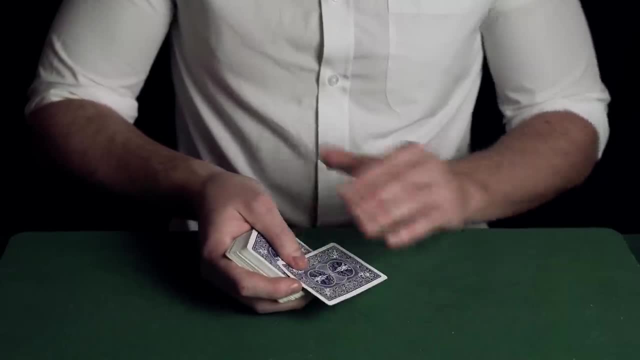 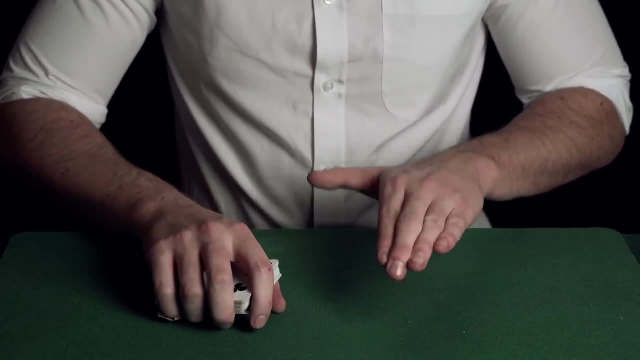 and as you do that, you pull the card flush with the rest of the deck and you vanish it like that, so at full speed. it looks very visual. i've got a full tutorial on this on my channel as well. i'll leave a link down in the description. 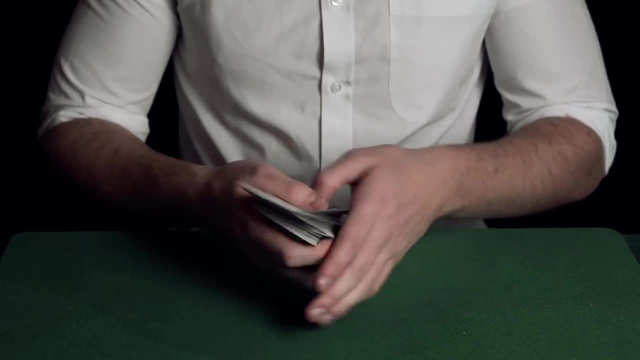 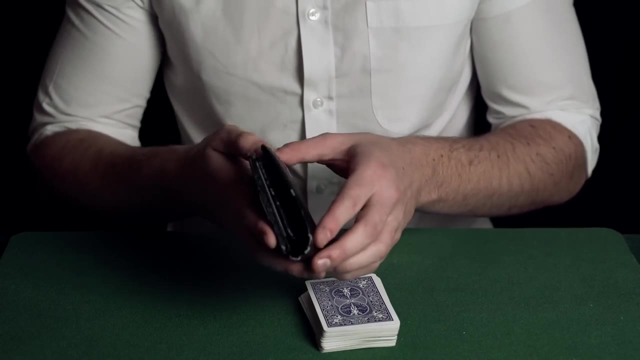 to where you can watch it. once you've made the card vanish, what you then do is you point to your pocket and say: the card jumped to the wallet. pull out your wallet and, instead of opening it to the main pouch, you open it to the fire pouch, which 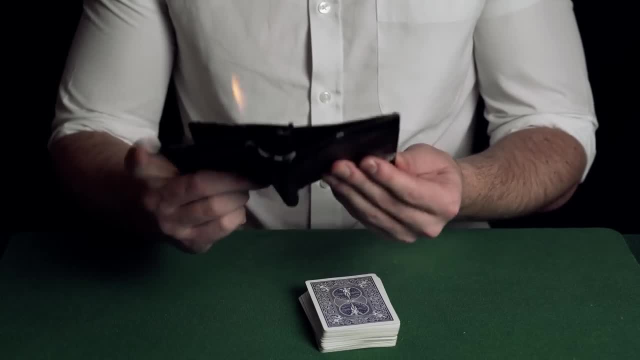 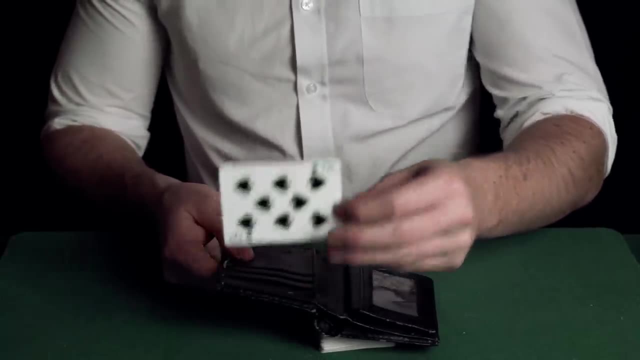 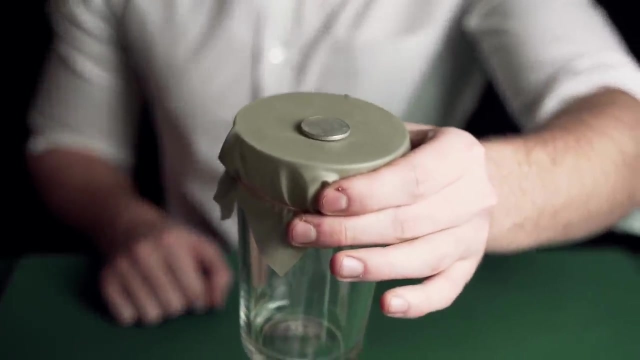 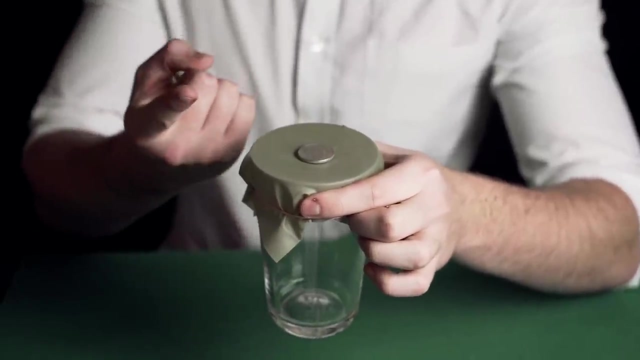 closes shut like this. you then just simply flick the switch. the fire appears, and then you close the flap and reveal the card. the magician places a coin onto some rubber and a glass. he shows it to the spectator. he then tells the spectator to take their finger and push the coin through the rubber. the spectator pushes down. 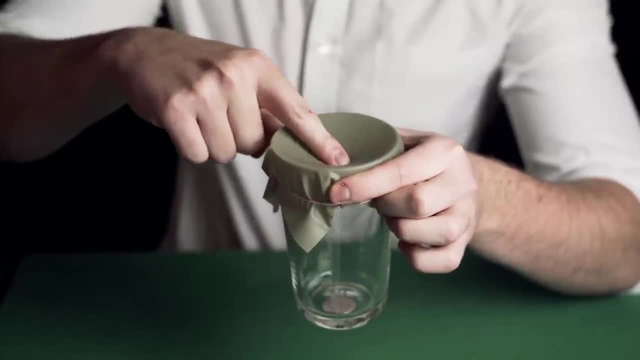 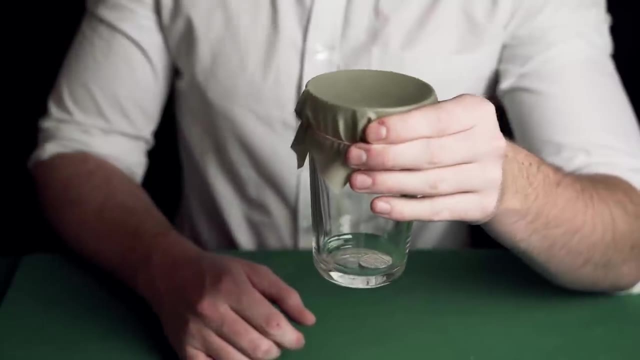 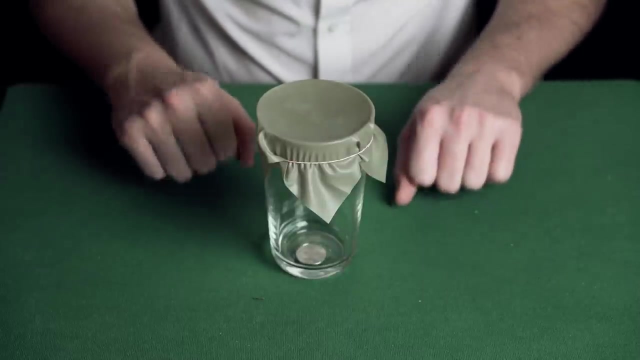 on the coin and it goes straight through the rubber. this is easily one of the best, most visual tricks ever created. everything can be inspected and there's absolutely nothing to hide. what's even better is that you can learn this in five seconds. you will need this special magic rubber.